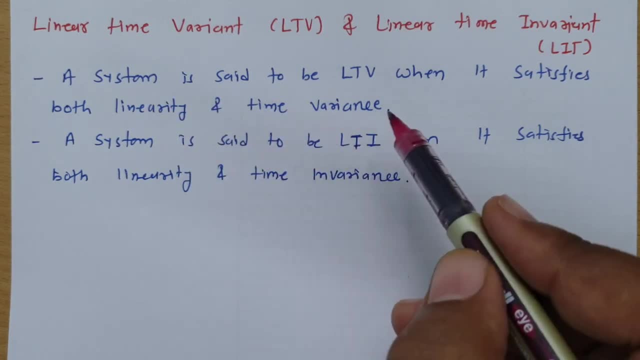 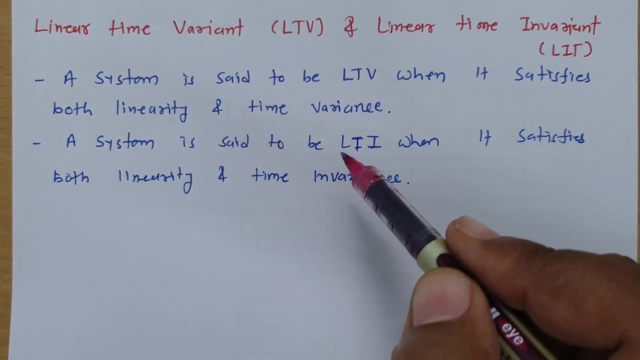 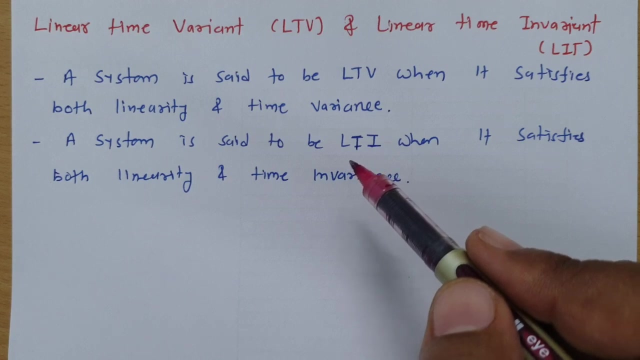 So if system is satisfying linearity as well as time variance, in that case it will be LTV. So if system follows linearity as well as time invariance, in that case we can say: system is linear, time invariant system, LTI system. 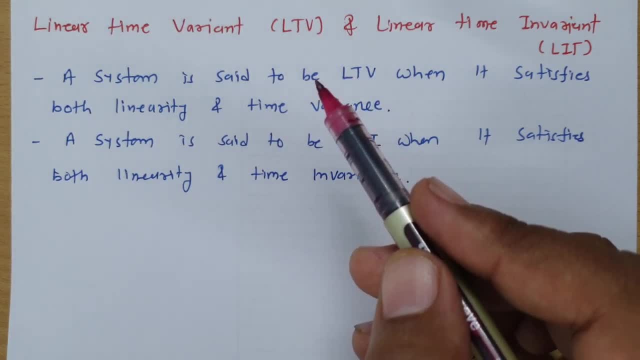 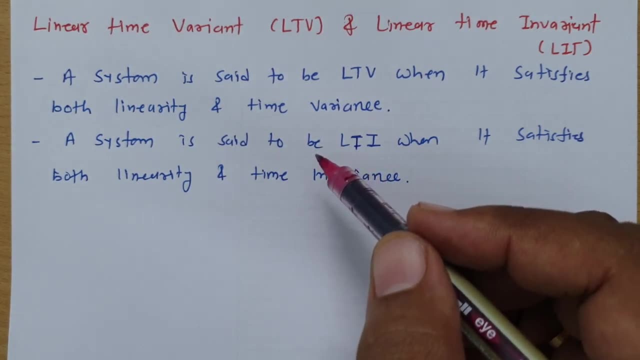 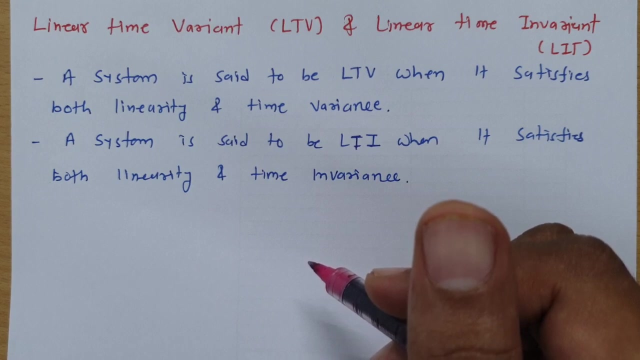 So when we try to calculate whether given system is LTV or LTI- linear time variant or linear time invariant- in that case we need to check both of these conditions- linearity as well as time variance- And based on that we can identify whether it is LTV or LTI, or both are there or not. 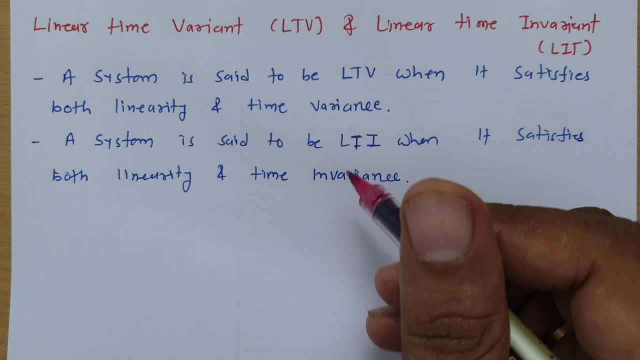 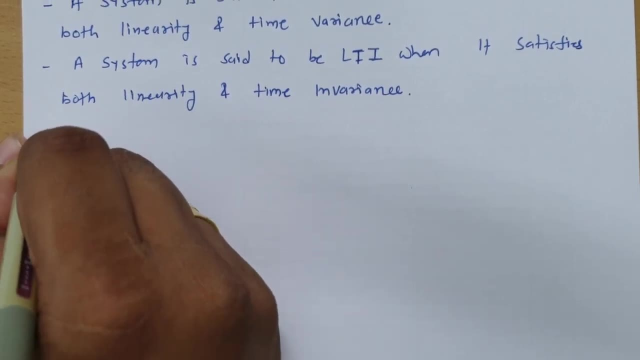 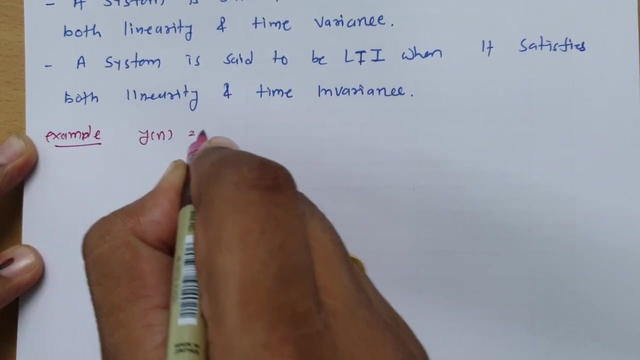 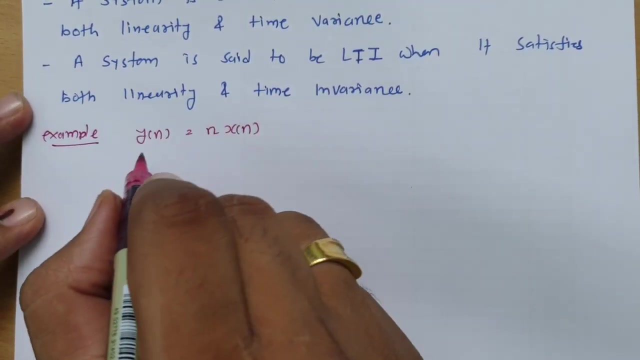 So let us try to understand this with one example, so it will be more clear. Now, see, I will be considering first example: If y of n, that is n into x of n, so first i will be checking linearity. so for linearity we need to calculate superposition. 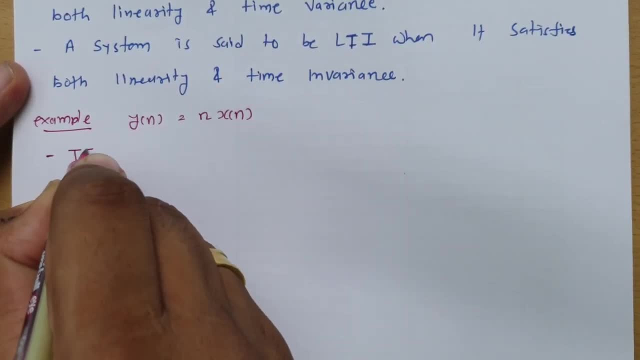 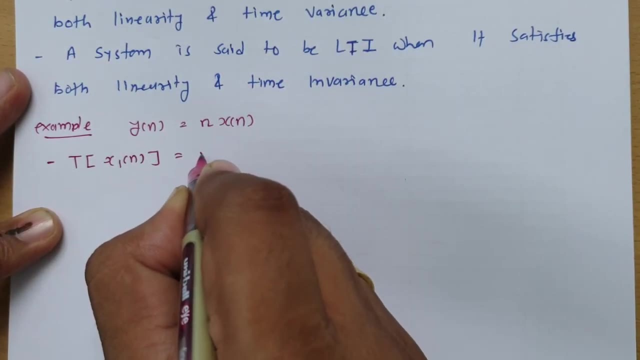 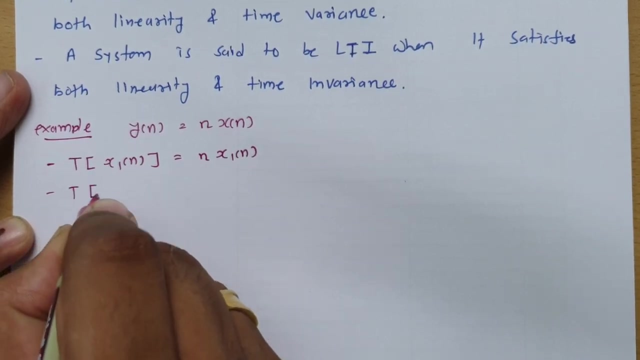 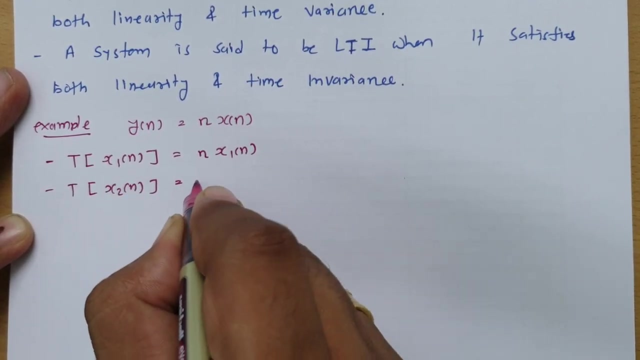 principle. so what i will be doing is i will be calculating first transpose of input is x1 of n, so in that case my output will be n into x1 of n, and if i calculate response, transpose of x2 of n. so in that case my output response will be n into x2 of n as y of n. 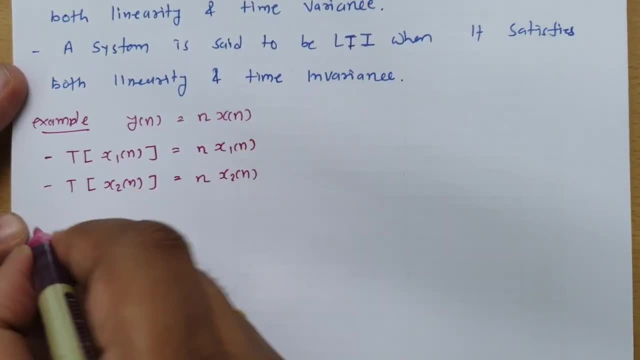 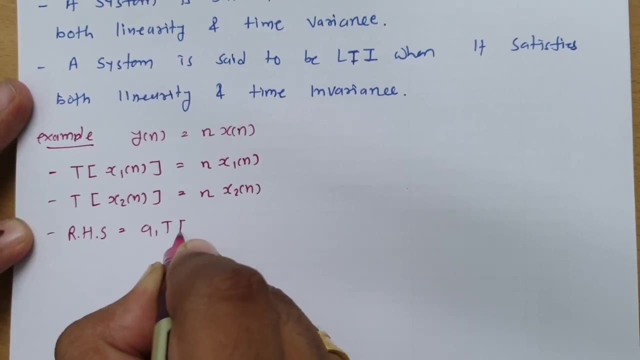 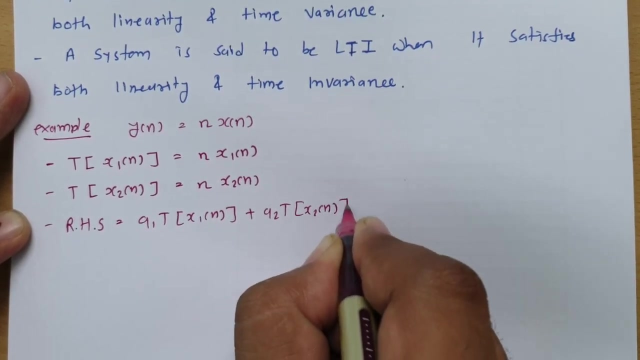 is equals to n into x of n. so if i calculate lhs, sorry rhs, so rhs is what a1 transpose of x1 of n plus a2 transpose of x2 of n. so if you place this value so that you will get the Bernstein equation, totally fine. 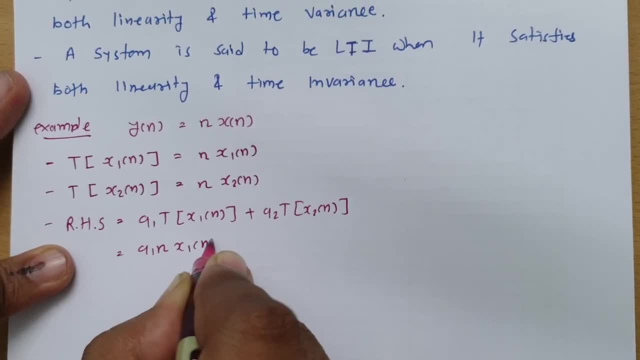 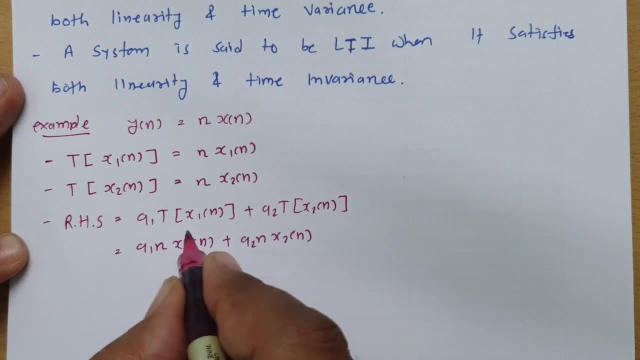 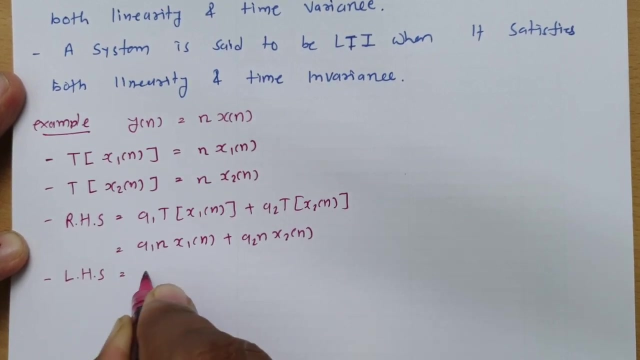 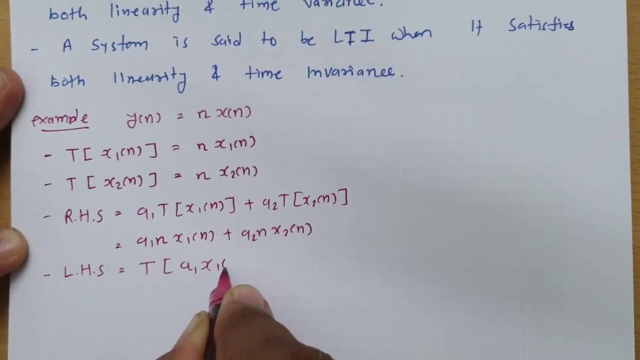 that will be a1n, x1 of n plus a2n, x2 of n. now if you combine this two signal so you can calculate lhs. so lhs, that is transpose of combined signal, that is a1, x1 of n plus a2, x2 of n. 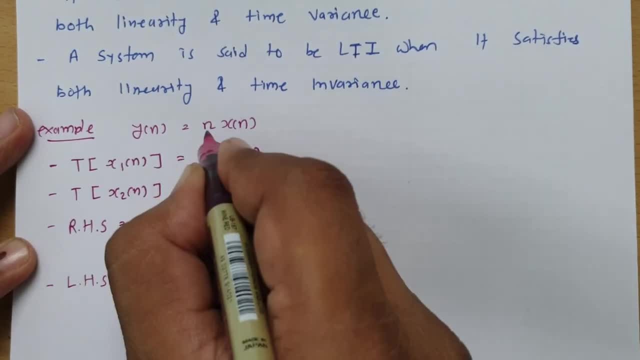 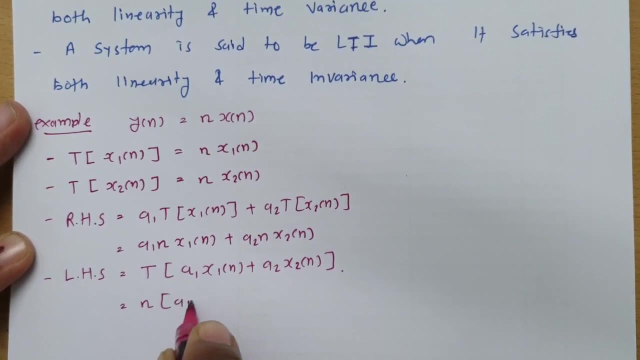 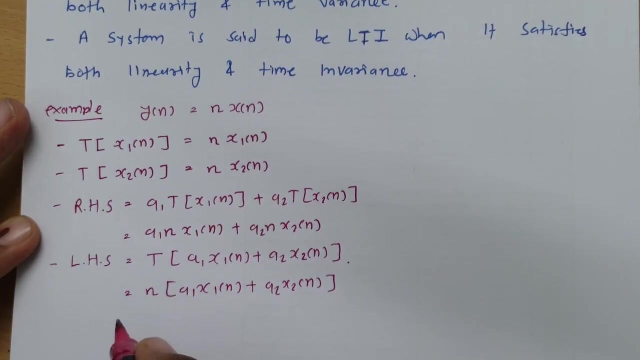 so in this case you will be finding n will be as it is and instead of x now it will be combined input signal, so that will be a1 x1 of n plus a2 x2 of n. so this will be practically a1 n- x1 of n. 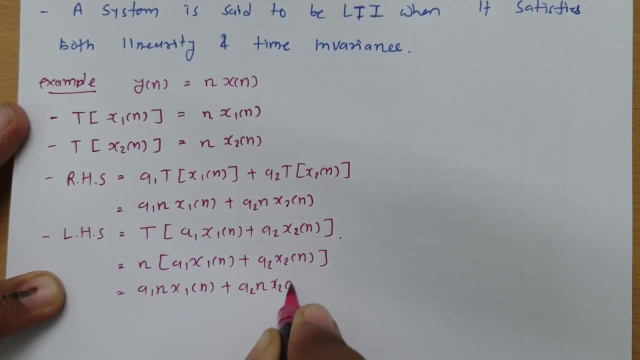 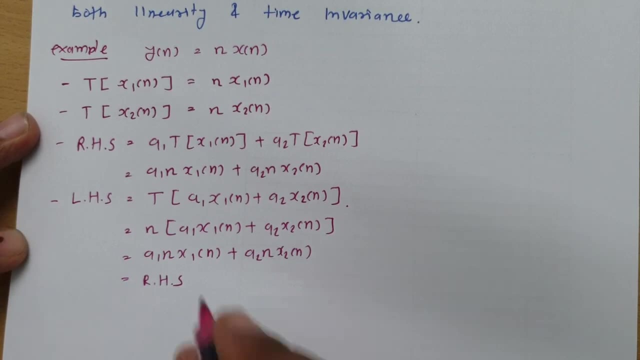 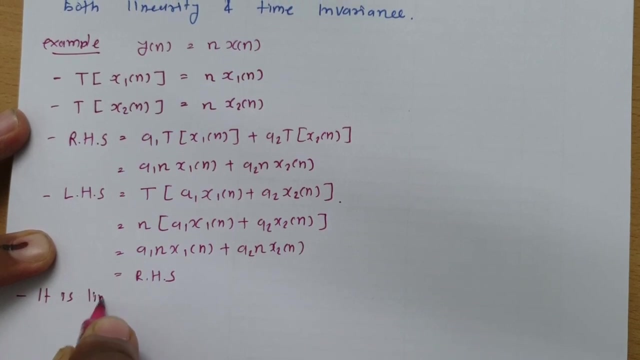 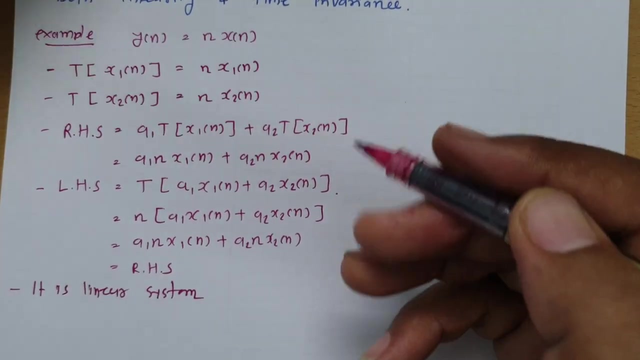 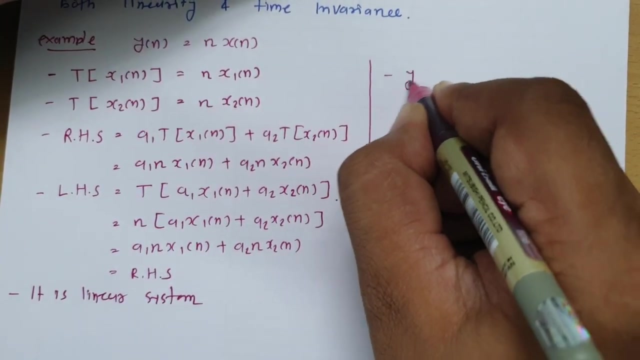 plus a2, n, x2 of n, and that is actually i lhs means given system is linear system. so it is linear system that we can say. based on this principle of linearity, now let us calculate time variance condition. so for that we need to calculate y of n comma k, so in y of n comma k. 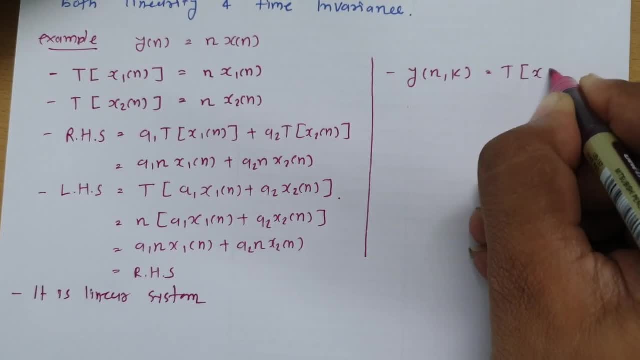 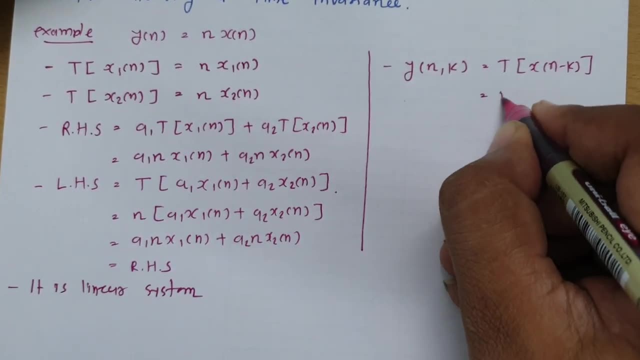 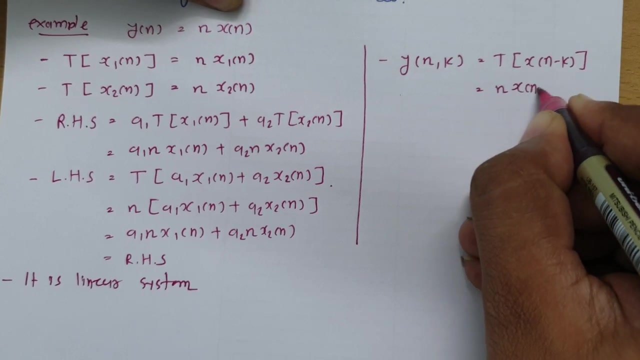 we need to calculate transpose of x of n minus k. so we need to replace x of n with n minus x of n minus k. so n will be as it is and x of n. now, this x of n that will change is to x of n minus k. 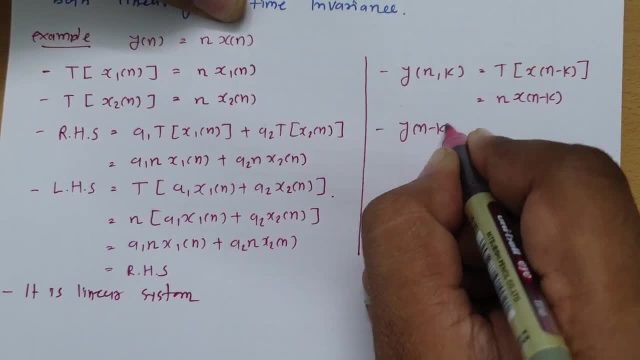 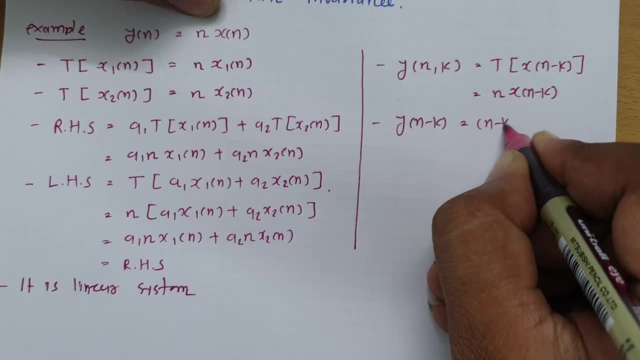 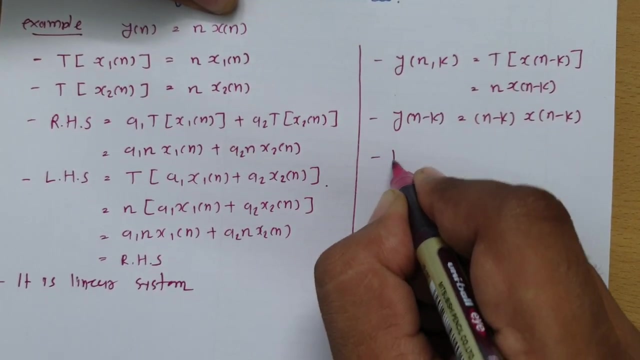 and when you calculate y of n minus k, you will have to replace all n with n minus k. so here n is there, so that is n minus k. x of n minus k. that will happen. So we can say: here y of n comma k is not equals to y. 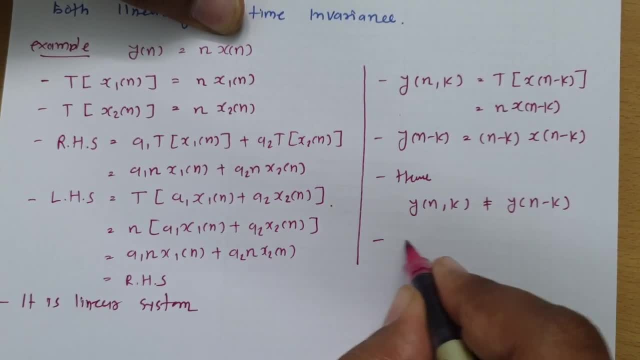 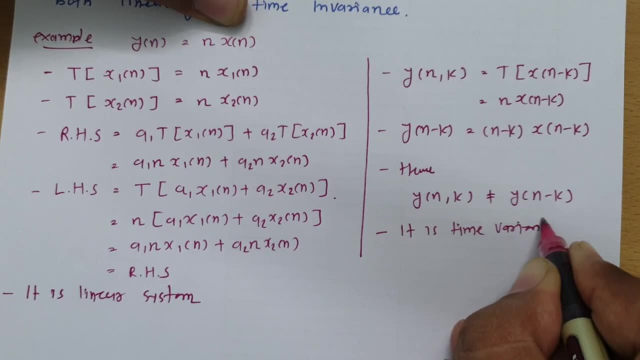 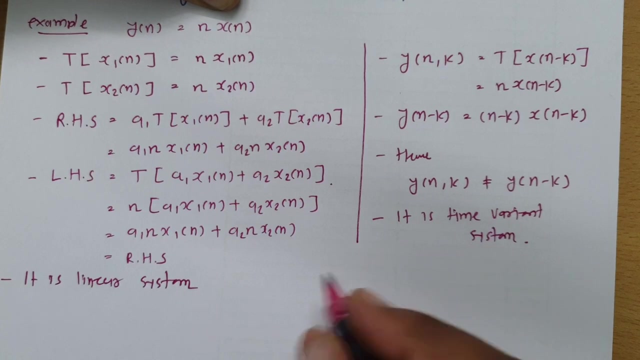 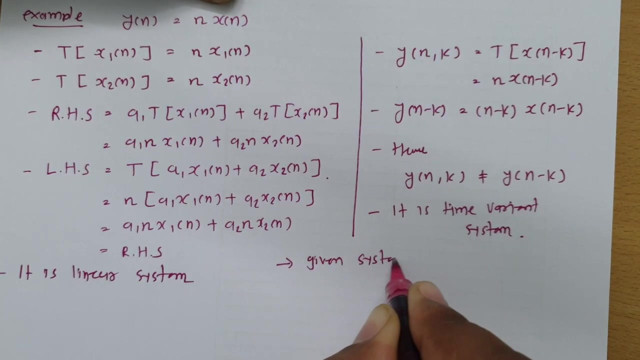 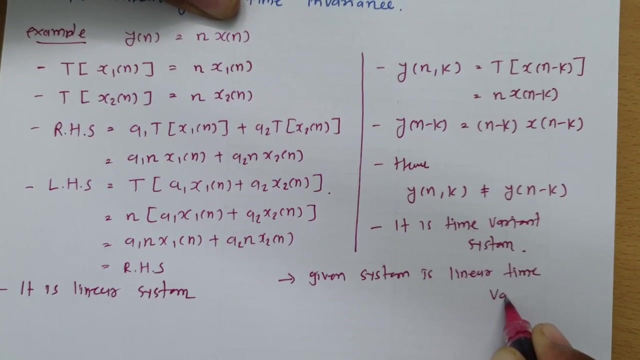 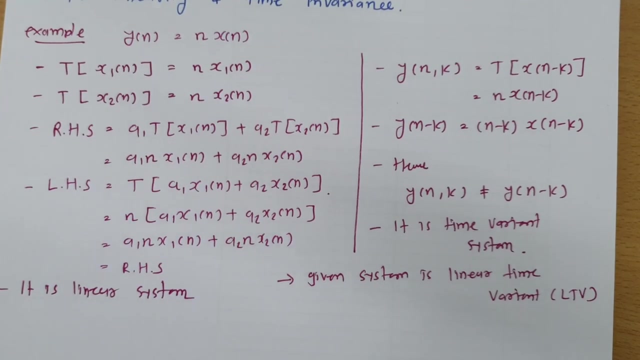 of n minus k. So this system, it is time variant system. So we can say: this system is linear as well as time variant system. So from both we can say: given system is linear, time variant means LTV system. It is linear time variant system. Now let us have one more example. 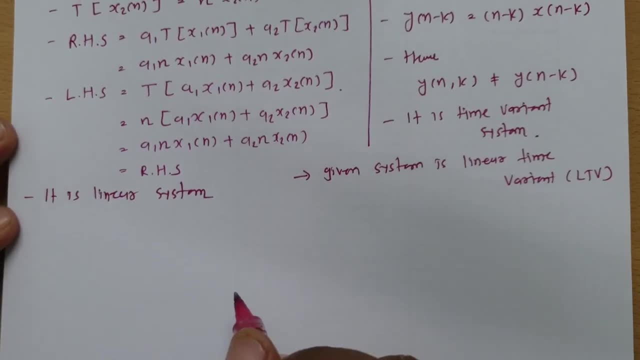 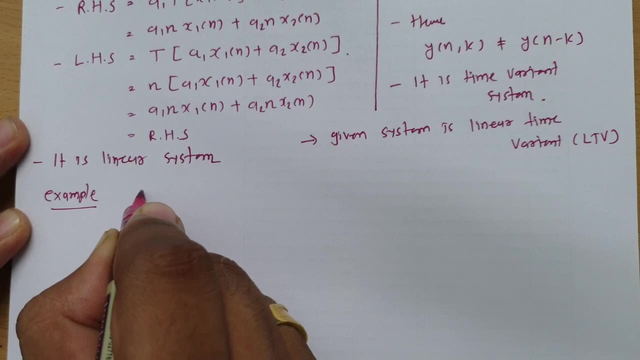 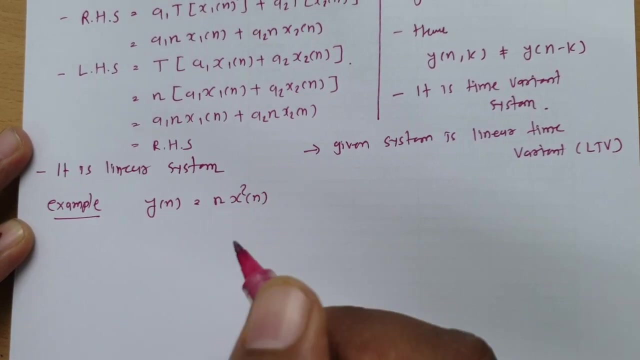 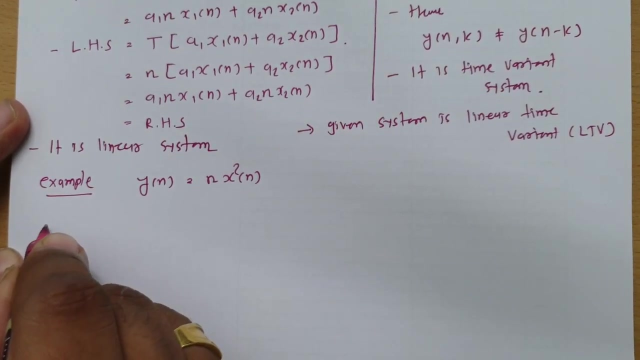 So it will be more clear. So now I will be considering a case y of n that is equals to n into x square of n. Now let us identify linearity first. So for linearity, I need to check response with. 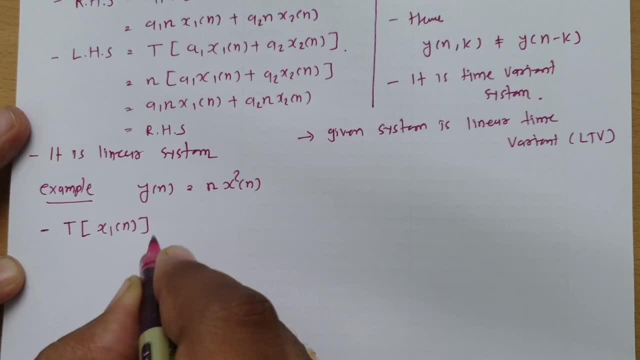 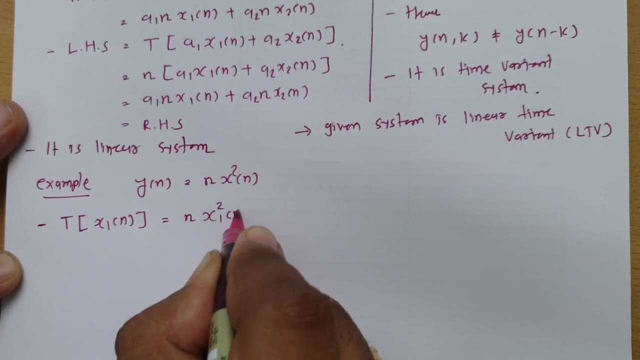 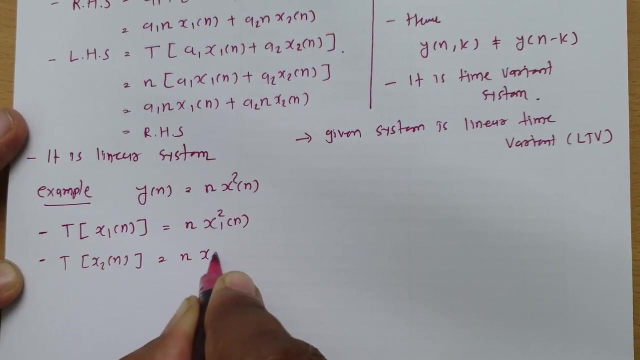 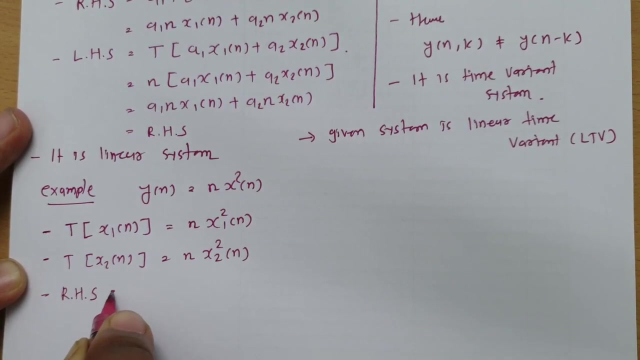 input x1 of n, So transpose of n- So that is n- into x1 square of n and transpose of x2 of n, So that is n into x2 square of n. So from this we can calculate RHS. So that is a1 transpose of x1 of n plus a2 transpose. 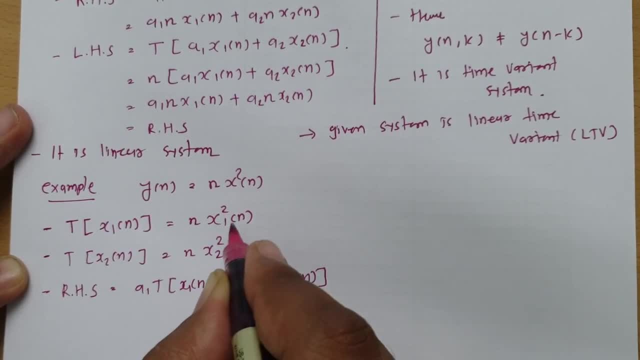 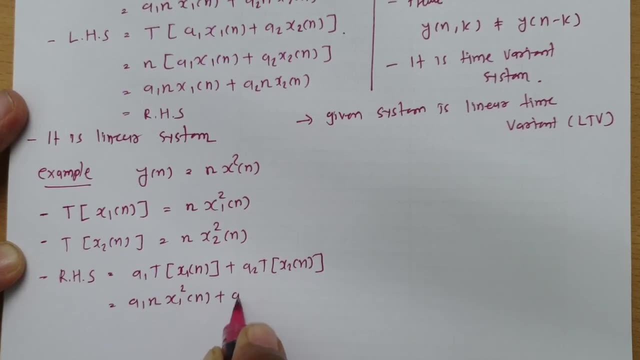 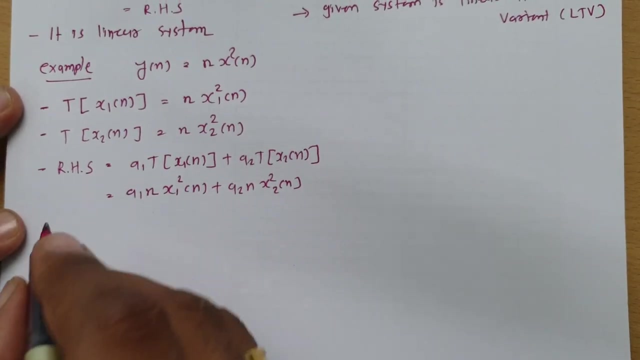 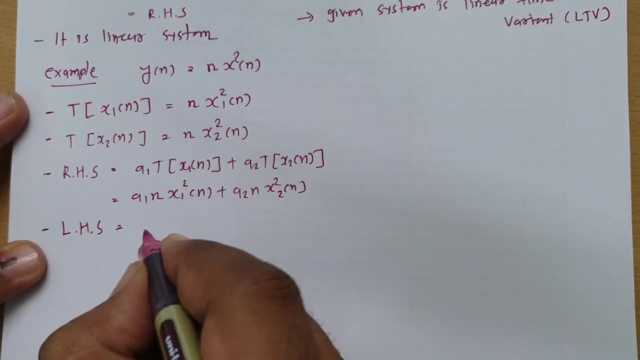 of x2 of n. And if you place this two values you will be getting it is a1n x1 square of n plus a2n x2 square of n. Now for linearity: RHS. that is what combined signal. So now combined. 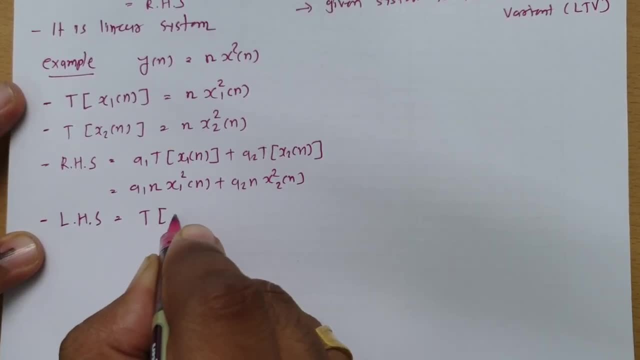 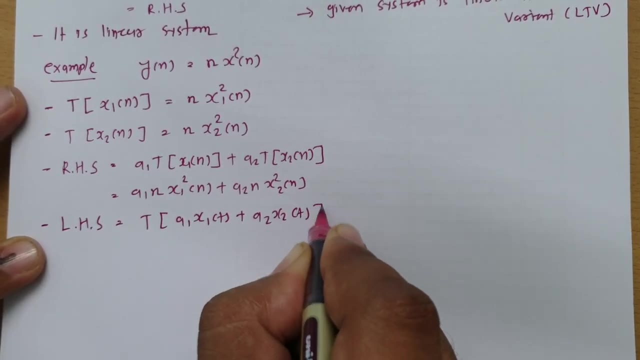 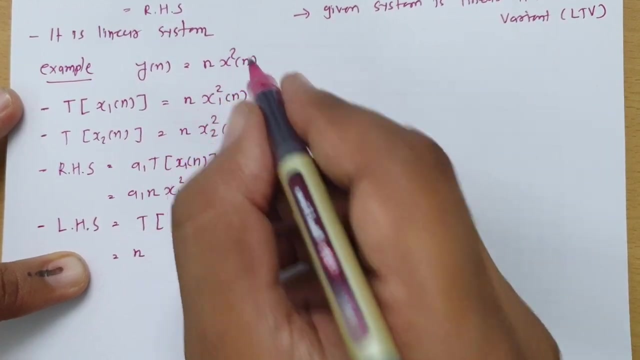 signal will be transpose: response of a1- x1 square of n. So this is the linearity of it: t plus a2- x2, t. So that will be now n as it is, and output is square of x1- x. So here input. 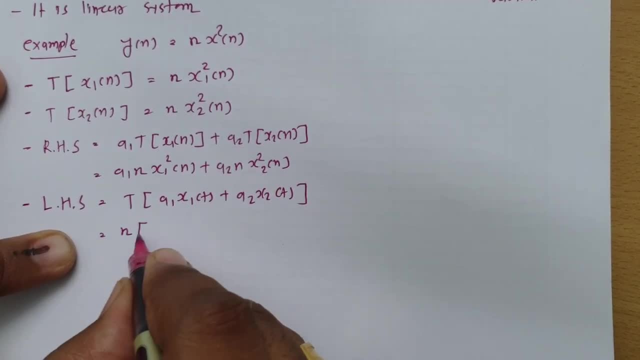 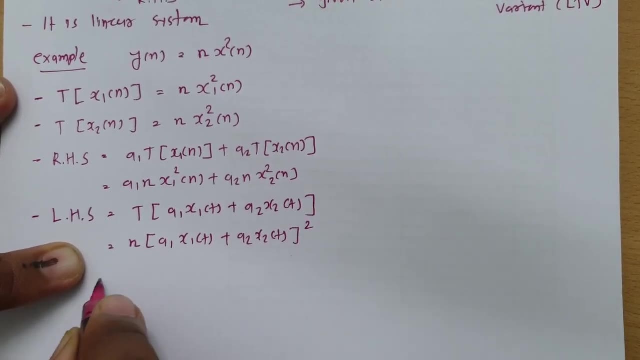 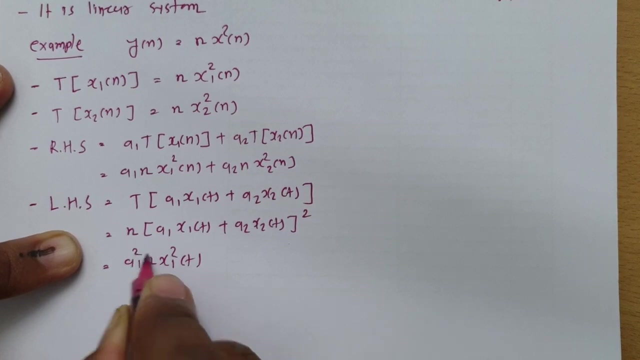 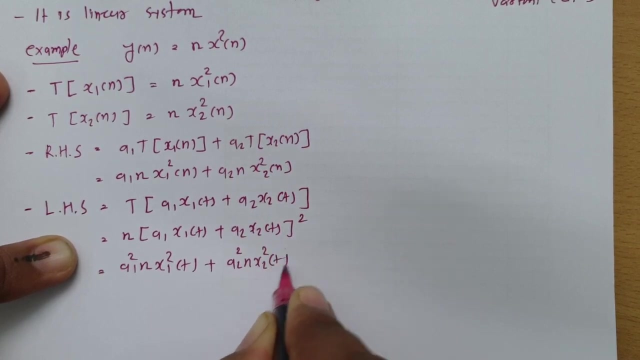 is a1 x1 t plus a2 x2 t, So square of this a1 x1 t plus a2 x2 t, whole square. So this is a1 n x1 square of a1. square n x1 square of t plus a2 square n x2 square of t plus. 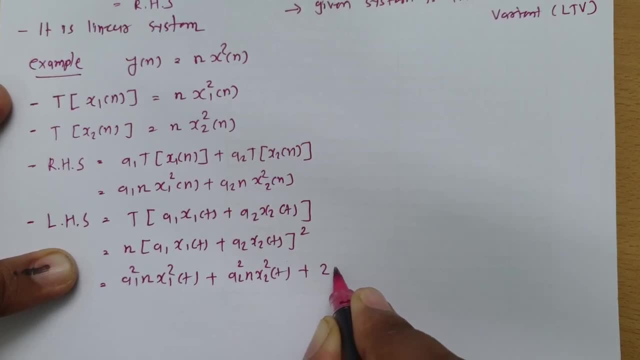 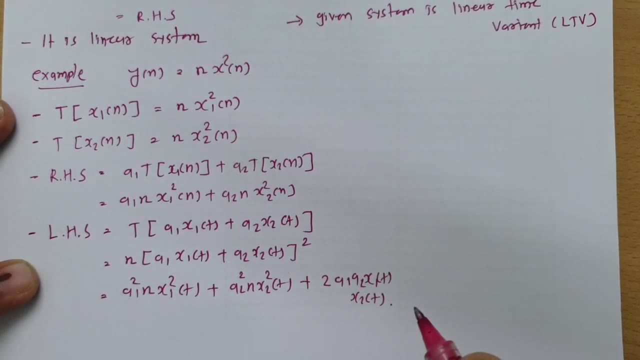 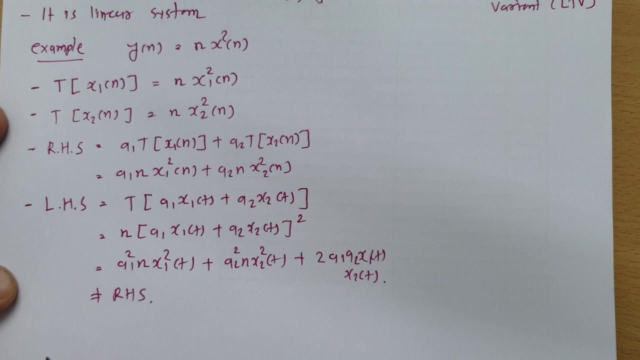 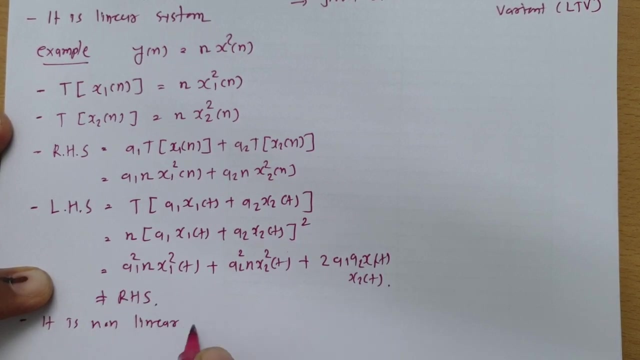 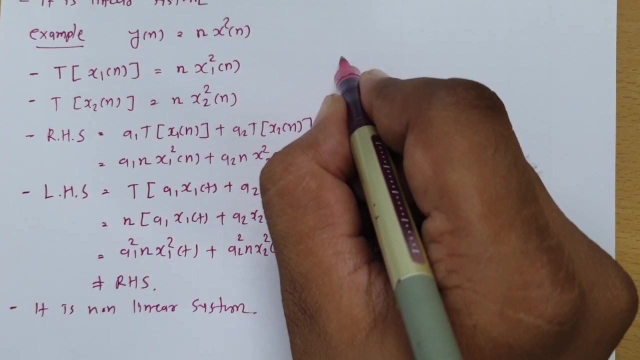 2, a1, a2, x1 t, x2 t. So this is not equals to RHS. So as this is not equals to RHS, we can say it is non-linear system. This is non-linear system Now if we calculate time variance property. So for that we need to calculate. 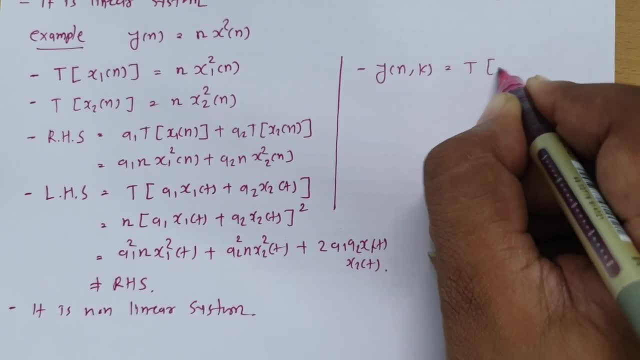 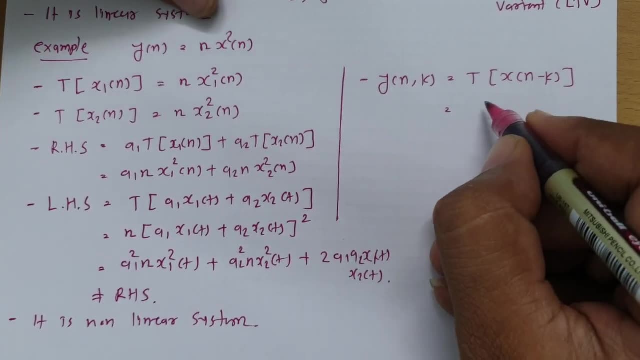 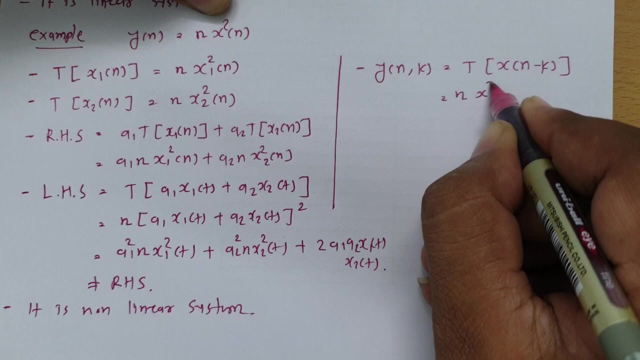 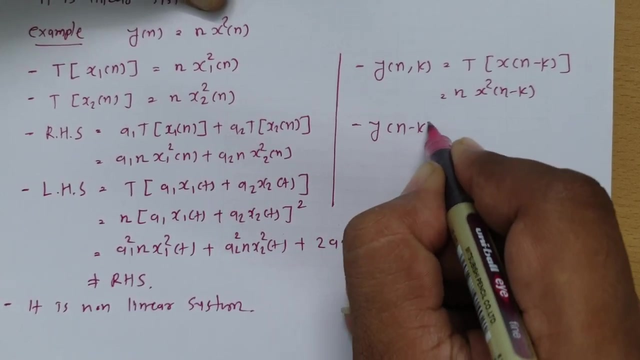 y of n comma k, and that is transpose of input, x of n minus k. So we need to calculate y, to calculate only, we need to change only input. so n will be as it is and x of n that will change is to x square of n minus k. and if you calculate y of n minus k, so in that case we need to replace: 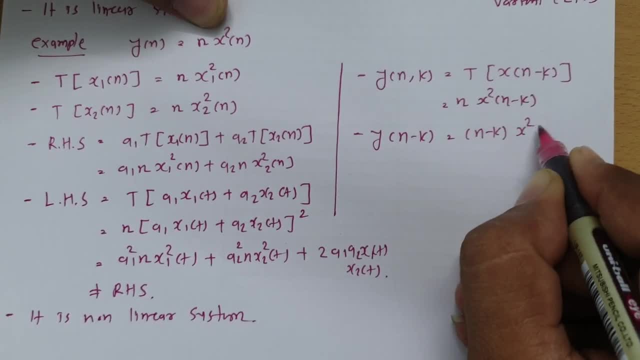 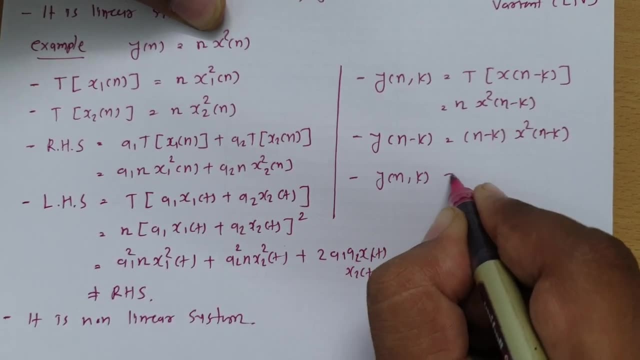 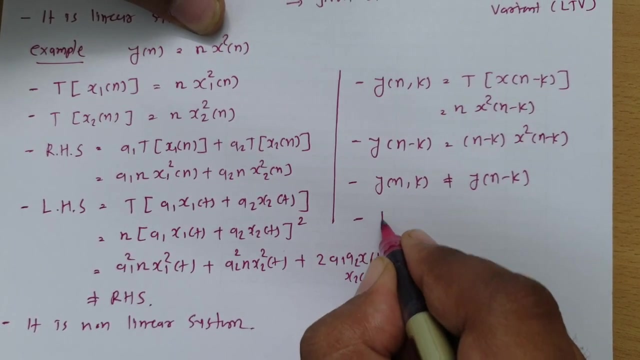 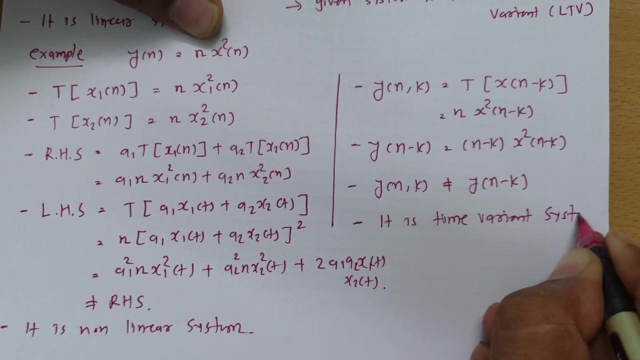 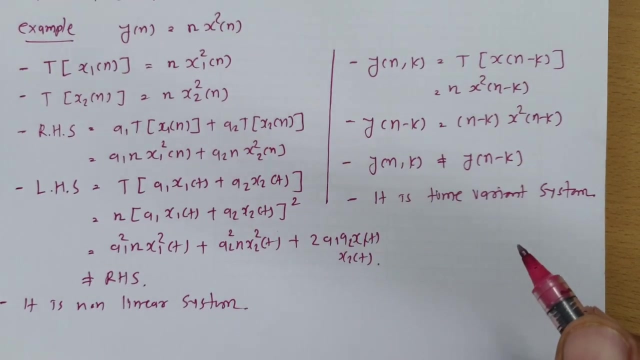 n with n minus k, so n minus k into x square of n minus k. so here one can observe: y of n comma k that is not equals to y of n minus k. so this is what time variant system. it is time variant system. so here this given system is non-linear and time variant system. so from this we can say: 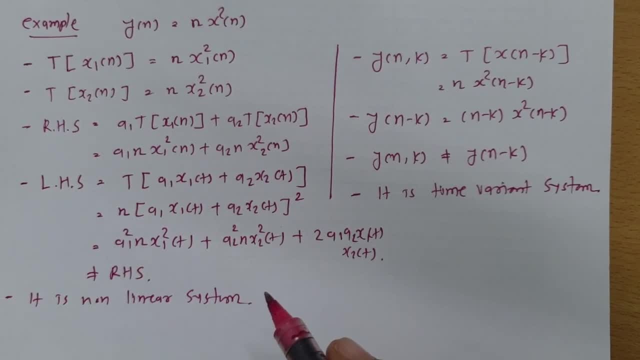 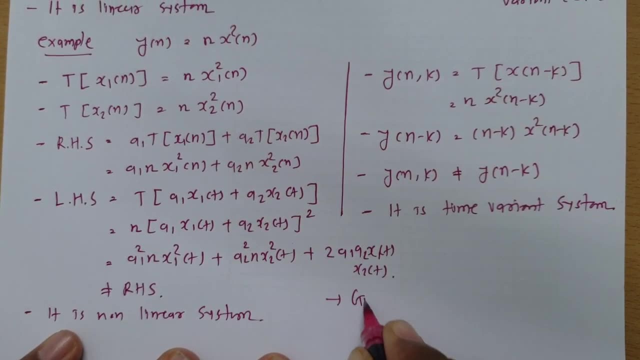 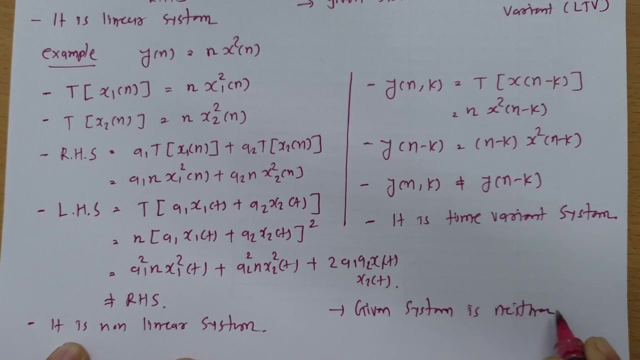 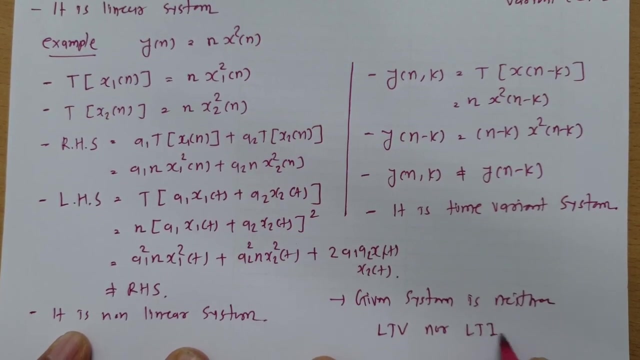 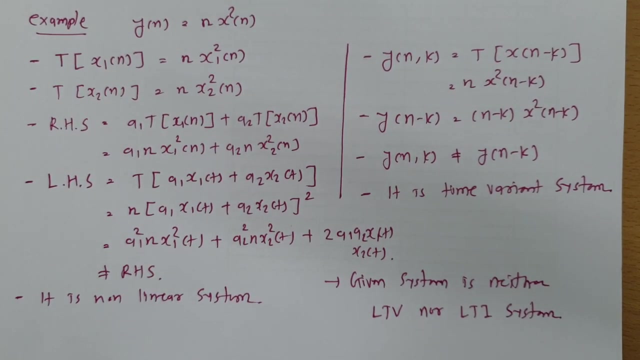 it is neither ltv nor lti system as it is non-linear system. so given system is given system is neither linear time variant nor linear time invariant system. so this system is not both. so this is even possible. so i hope that you have understood this: how to identify linearity and time invariant?